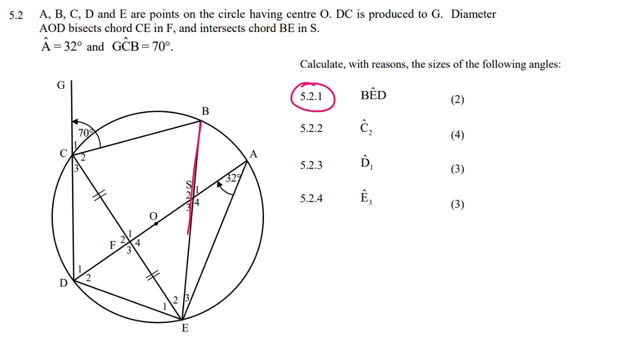 So BED. So if this is BED, Okay, so it's this entire angle over here. Now can you see the cyclic quadrilateral over there? Well, we know that the external angle of a cyclic quadrilateral is equal to the inside opposite angle, And so immediately we can say that angle BED. 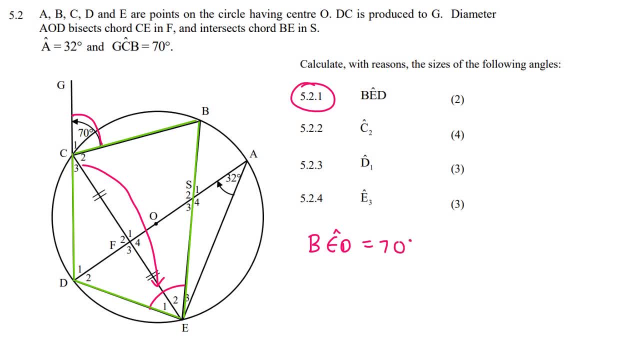 is equal to 70 degrees because of external angle cyclic quad. Moving on to question 5.2.2, where they want to say: how do you calculate the angle of BED? So BED is equal to 70 degrees because of external angle cyclic quad. Moving on to question 5.2.2, where they want to say: 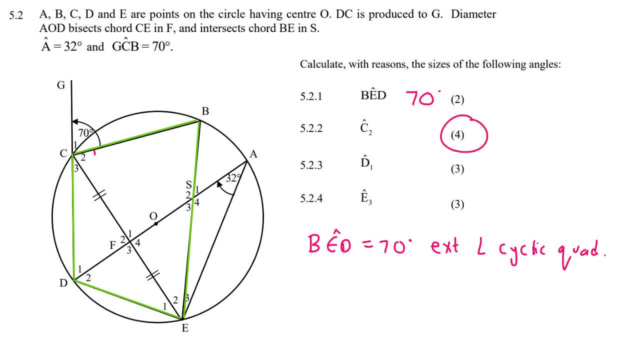 how do you calculate the angle of C2 for 4 marks? So what I noticed when I was looking at this was that there is a bow tie. You know the bow tie that you wear when you go to a, when you're wearing a. 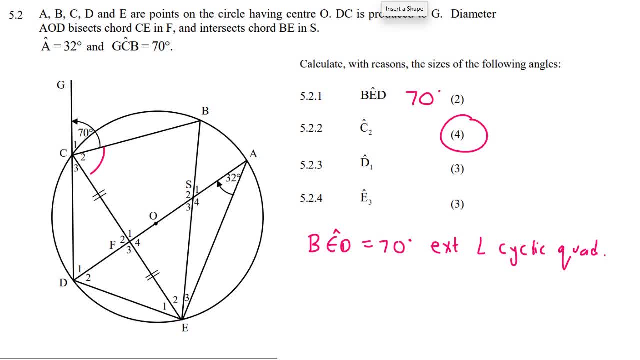 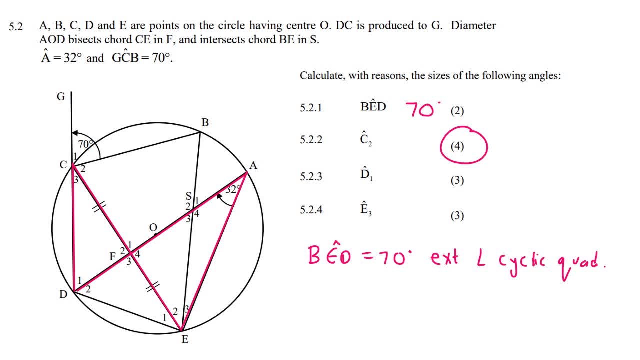 suit, for example, and you have a bow tie. Well, here it is, over here. So whenever you see a bow tie, that is a good sign, because it means you're going to be able to find some angles. If I show you a normal bow tie like this, you must remember that the top angles are always the same. 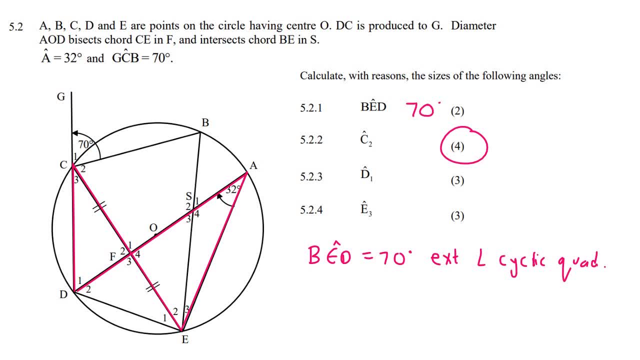 and then the bottom angles are the same, And so what that means for us is that these two angles are the same and these two angles- let's do that in a different color to show that they are different, like that, So we can instantly see that this is 32 degrees. So that means C3 is also 32. 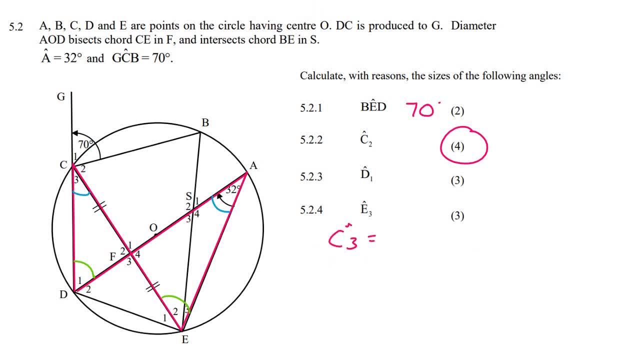 degrees, So C3 is 32 degrees, and that's don't call it the bow tie, It's called angles in same segment, And so we haven't found C2.. That's what we're really trying to find, but that's okay. 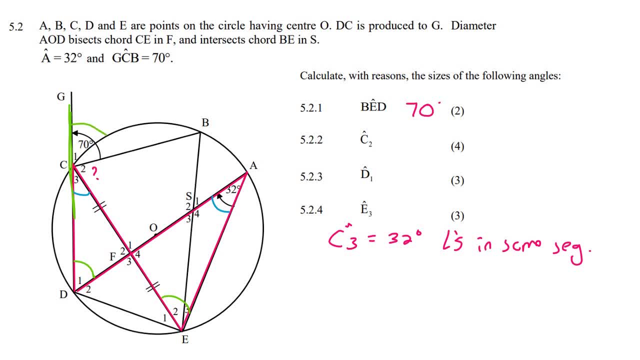 because here we have a straight line, And so we know that these three angles must add up to 180 degrees. So we can then say that angle C2 will be 180 minus 32 minus 70 degrees, And that's just because of angles on straight line, And so we could then calculate C2 as 70,. 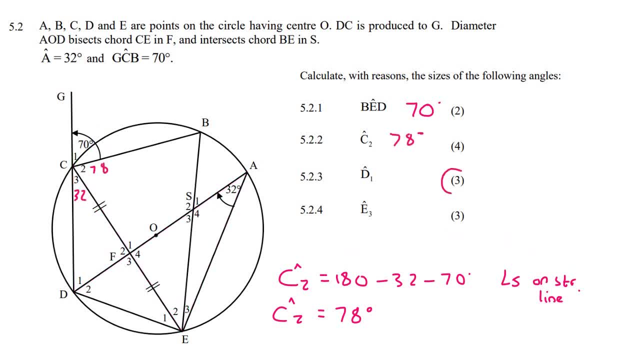 80 degrees. Moving on to the next question, for three marks, calculate the value of D1.. Here's D1 over here. This is very interesting, but can you remember one of the first circle theorems that you would have learned about is when you have a circle with a center and you have a chord. 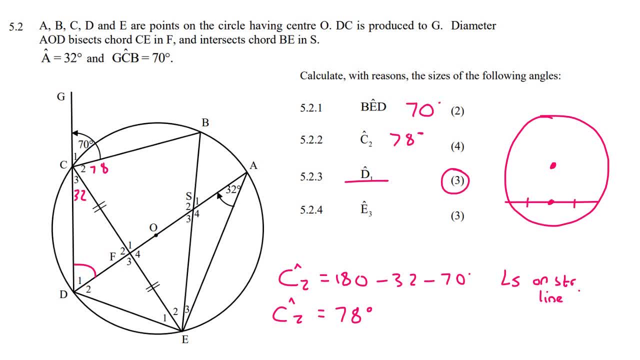 if you have a midpoint and you connect a line to that midpoint, then what does it automatically do? Well, well done. if you remember that it makes a 90 degree, Can we see that over here we've got a center of a circle, we have a chord over there and we have the midpoint. So what that means is: 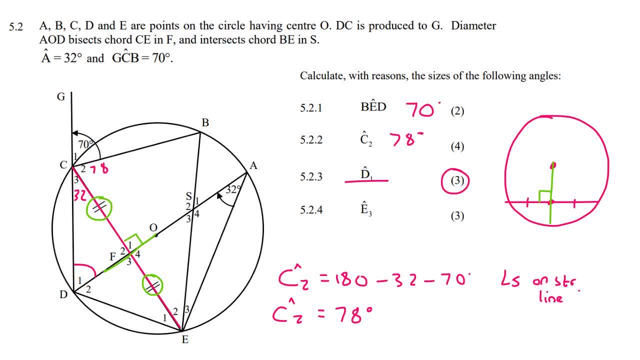 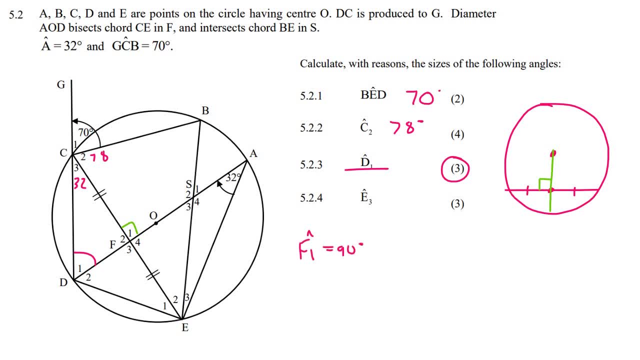 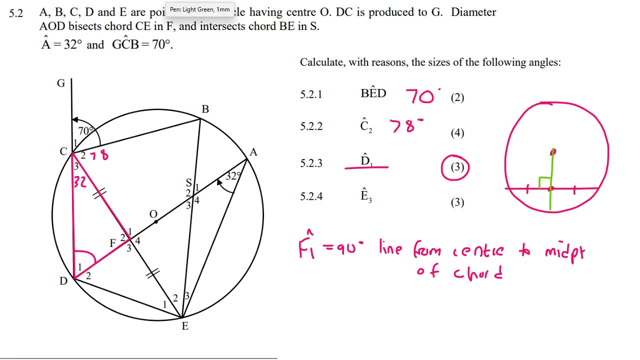 that this angle is naturally 90 degrees. So we can say that angle F1 is equal to 90 degrees because of line from center to the midpoint of chord. Now what we can do is we can work on the triangle that I've highlighted And that would easily 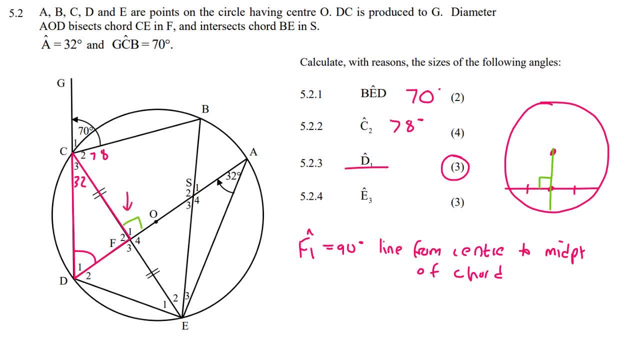 allow us to get to D1.. We could easily calculate D1 by working on this triangle. Now some students like to use. the exterior angle of a triangle is equal to the two interior angles, but a lot of students aren't very comfortable with that, So I'm going to use the longer method so we can say that F2 is also going. 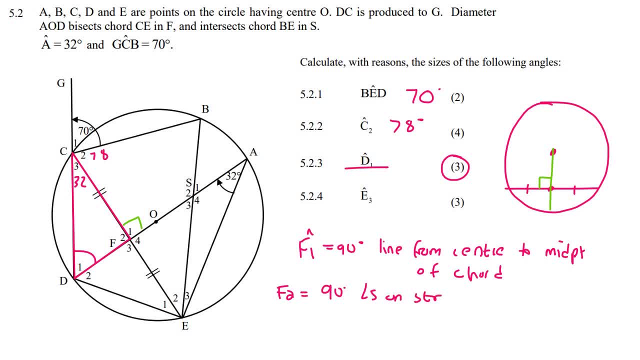 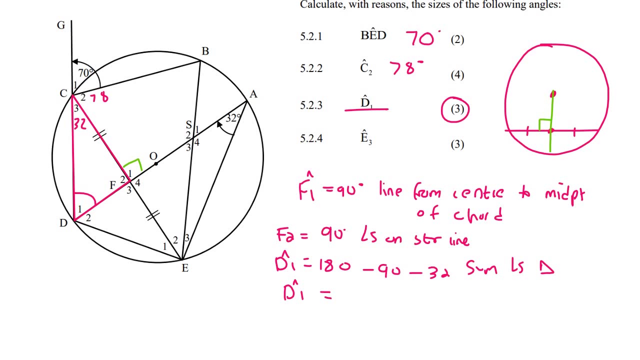 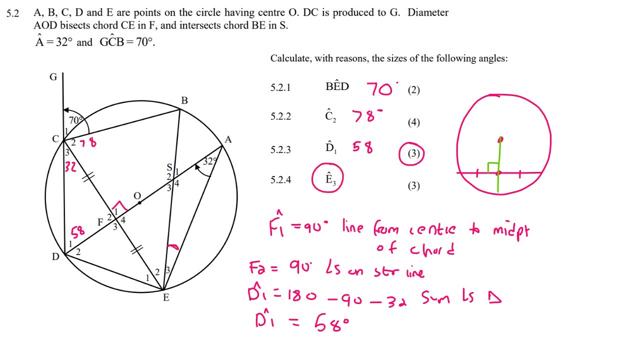 to be 90 degrees because of angles on a straight line, Then we can say that angle D1 will be 180 minus 90 minus 32 because of sum of the angles in a triangle, And then we would find out that D1 is equal to 58 degrees. And then the last question is E3. So E3 is over here Now. earlier on we 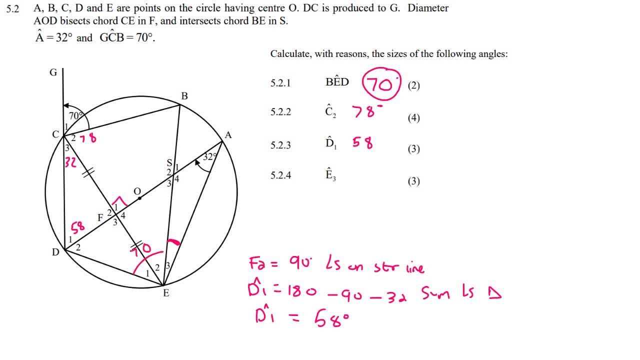 calculated that this angle was 70 degrees. Can you see that we have a diameter over here? Now, a diameter always makes a 90 degree angle. That is just because of angles in a semicircle. So we can say that angle D1 is equal to 58 degrees. And then the last question is E3. So E3 is over here. 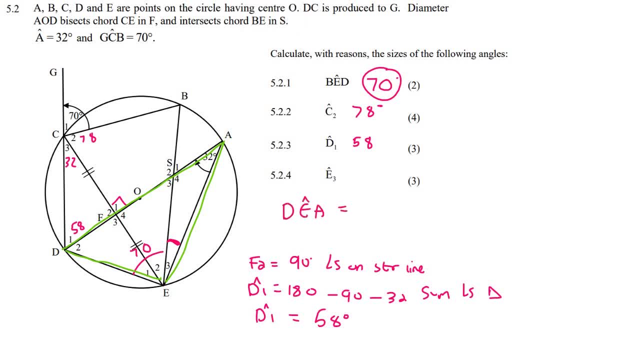 So we can say that angle DEA is 90 degrees, And that's because of angles in semicircle. So then, to find E3, we can simply say 90 minus 70, which would be 20 degrees.